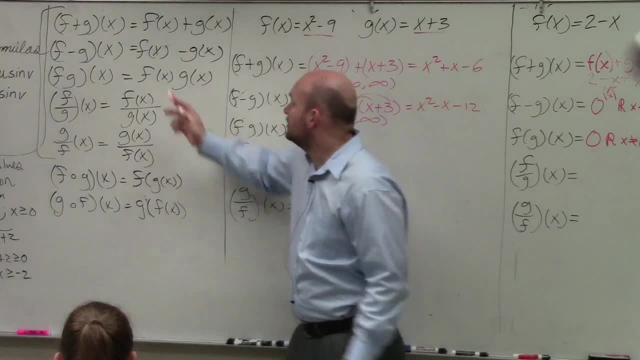 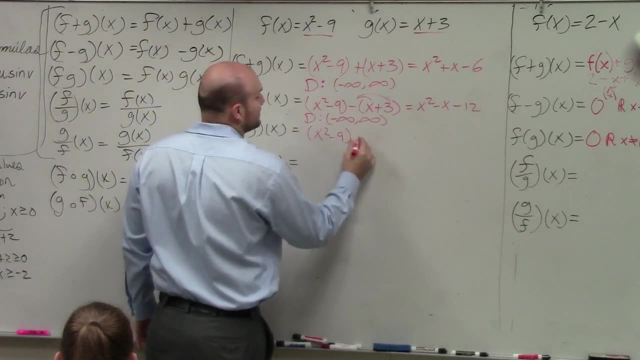 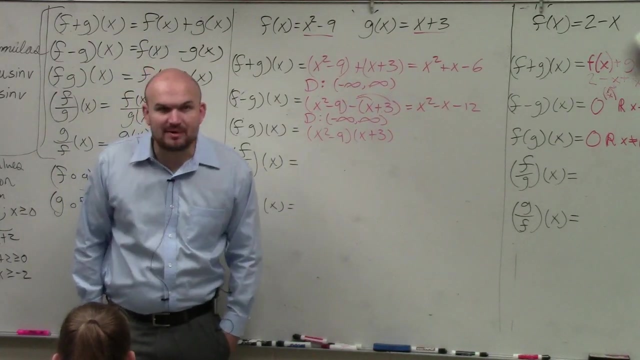 In the next example, you're multiplying. All it's saying is take one function and times it by the other function. All you guys had to do was do x squared minus 9 times x plus 3. And then distribute. Well, how do we know how to do this? We knew this by foil. 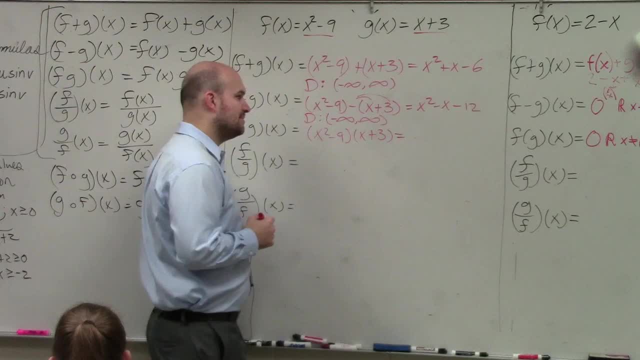 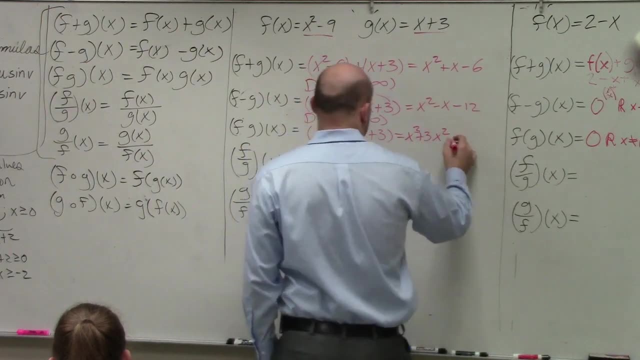 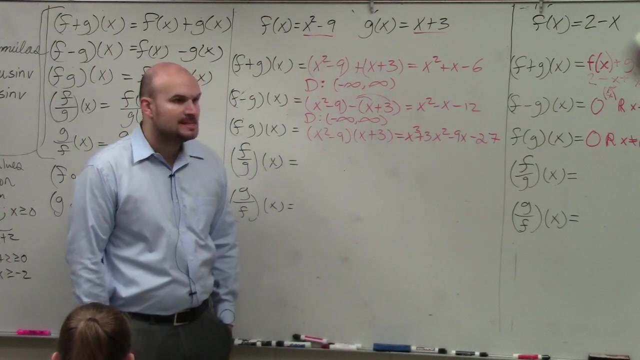 So by doing foil- I'll do foil in my head, but you guys might need to write it out- You'll have x cubed plus 3x squared minus 9x minus 27.. Are there any like terms I can combine? Nope, Is there? 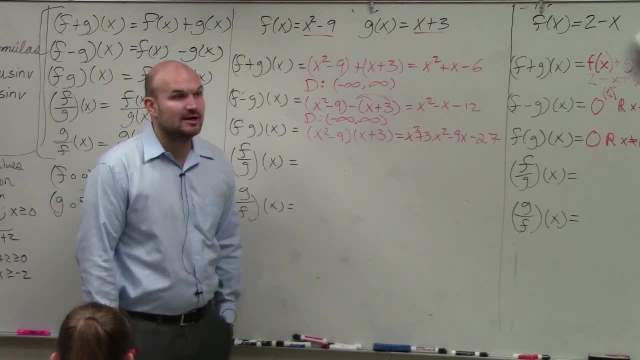 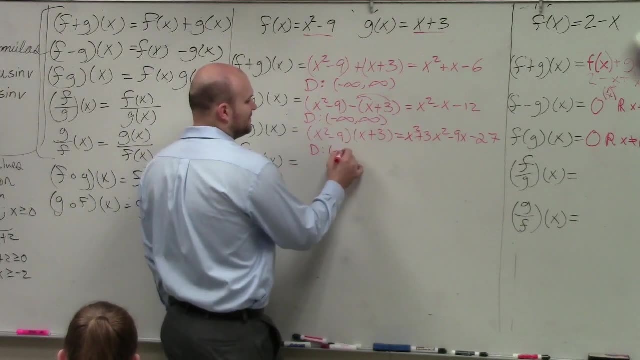 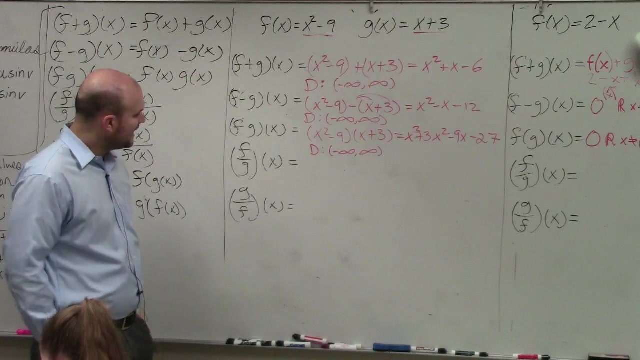 anything in the denominator. Is there anything in the denominator or in the numerator? No, So guess what? My domain is going to equal negative infinity In the denominator. I'll have g squared minus 9 over x plus 3.. We just like this own. that's everything in the denominator. 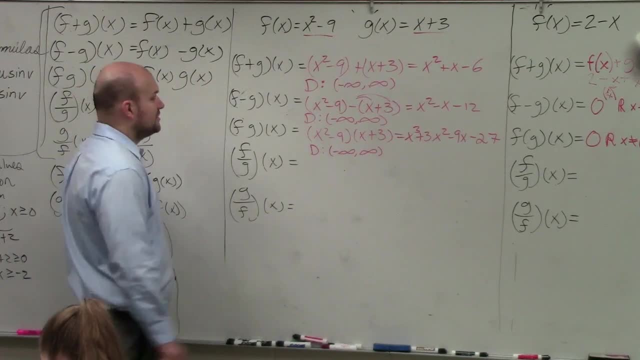 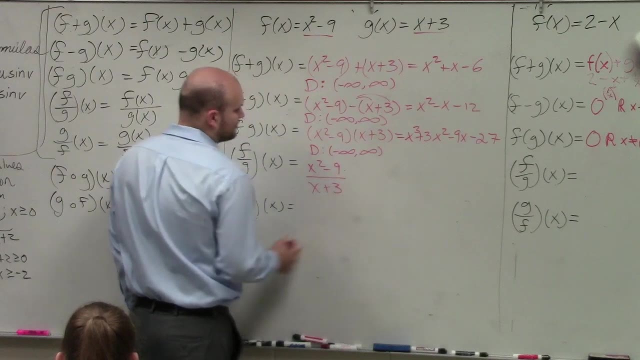 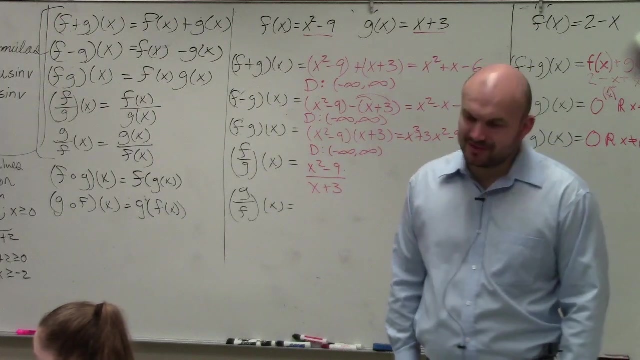 If I have, g equals 14.. aks, So I've got g equal 14 by 2 s squared over x And the denominator x cubed equals 9 times x squared minus 9x. Now let's go through this two during the course of the question. So instead of dividing over g, we're going to divide it by x. So let's go ahead and do this this way, And if we look at therah- we'll give it this- And at the answer that says: here we are going to divide f of x over g of x. 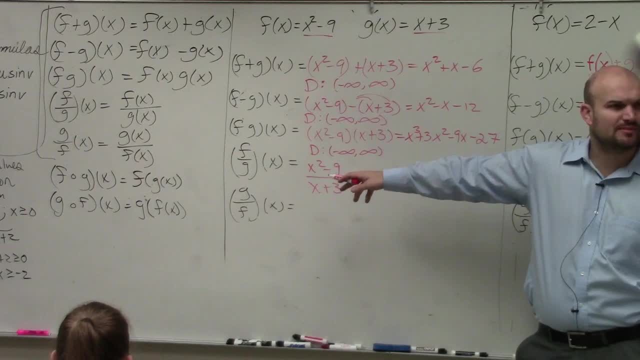 So I got x squared minus nine all over x plus 3.. Now I'm just going to- i'll give this table a little extra time. this time factor this: Can I simplify this at all: x squared minus 3? I can factor that into what? 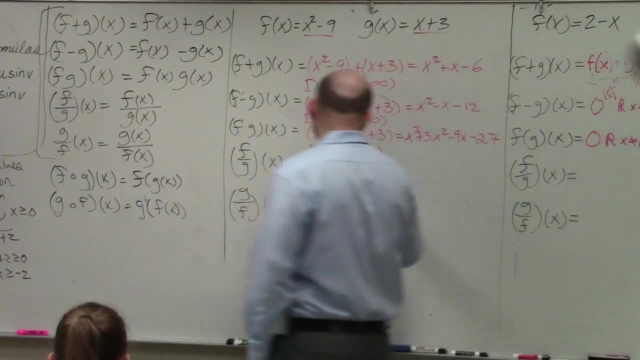 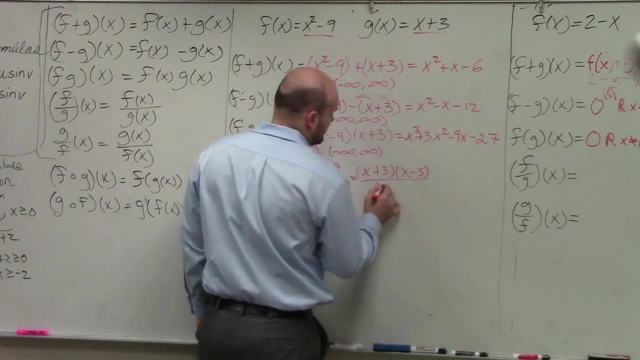 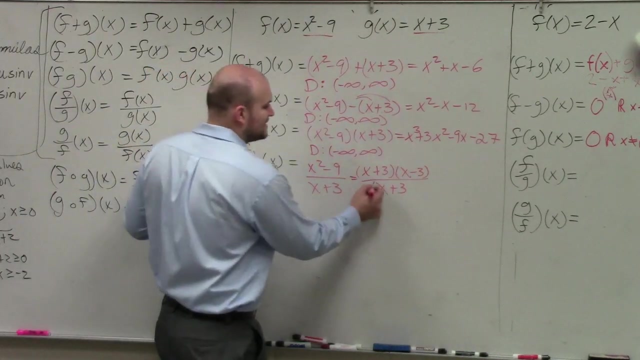 What can x squared minus 3 be factored to? And we'll learn about this later in the year, But when you have a rational expression and you need to simplify it, always look to factor that in. Therefore, then you guys see my x plus 3s can divide out. So my answer is: 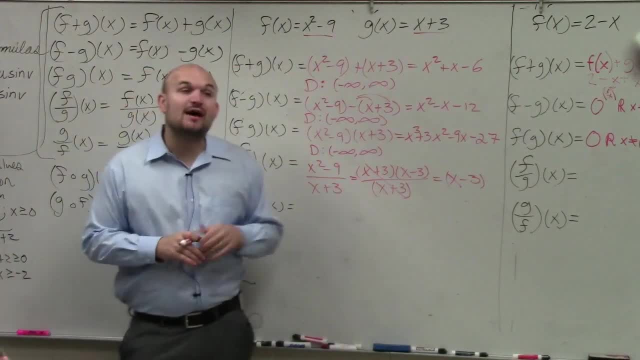 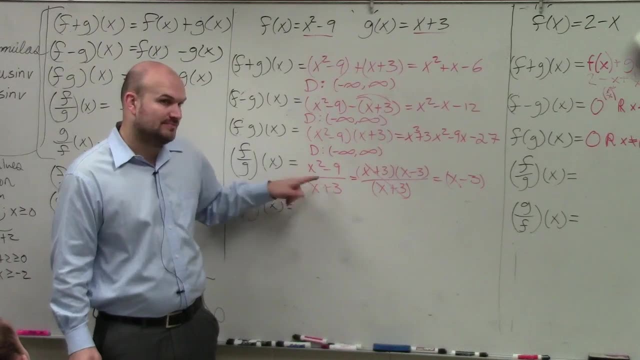 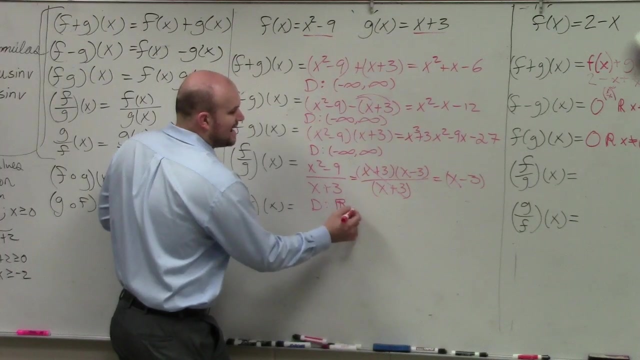 x minus 3.. However, when you are identifying the domain, your domain is still going to go back through your original function. You're going to use this original function, So my domain is going to be all real numbers, except when does 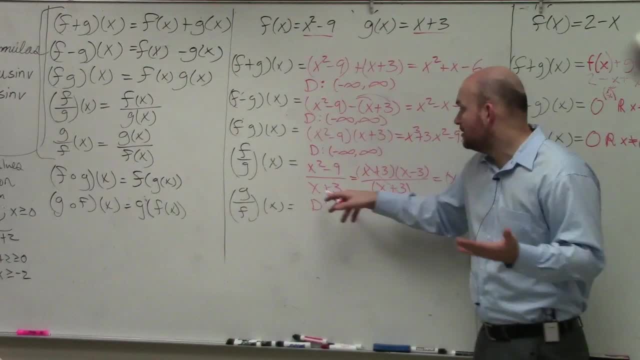 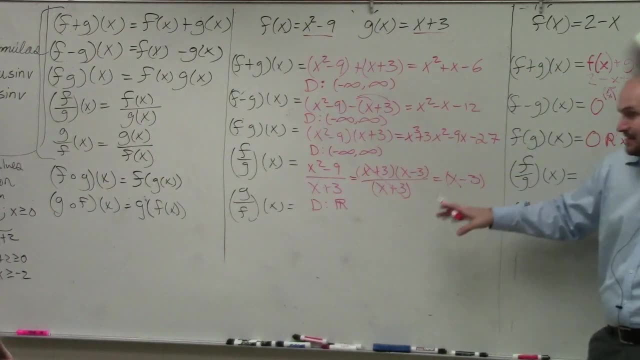 x. when does my? you guys noticed now. now we have a constraint, My denominator cannot equal 0. So when does my denominator equal 0 to my original problem? Don't worry about the simplified answer in this case, because we'll talk about this later. 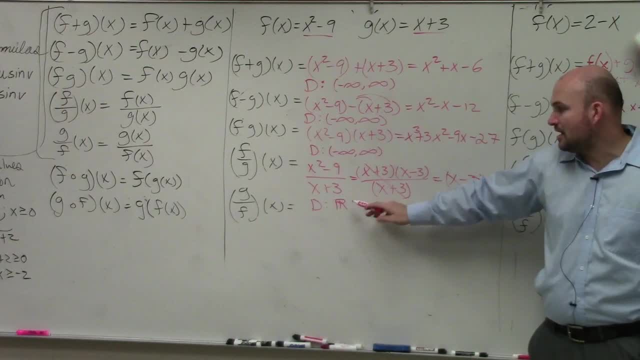 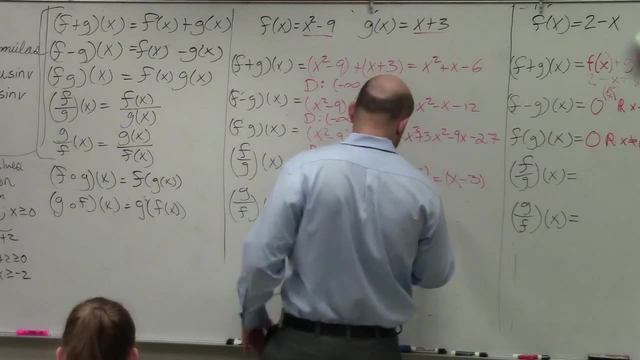 This is actually going to produce a whole. When does my range- I'm sorry, when does my domain equal 0?? For what values does that make it equal 0?? Nope, 3 plus 3 is 3.. x plus 3 equals 0.. 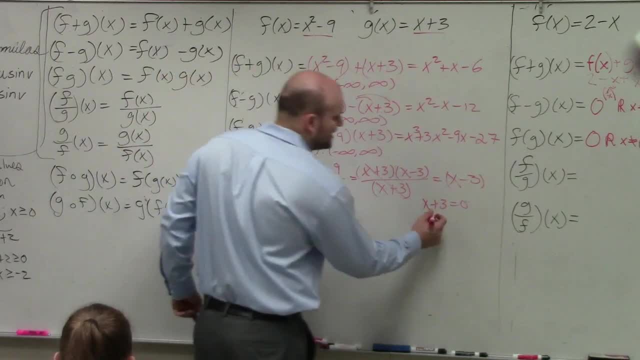 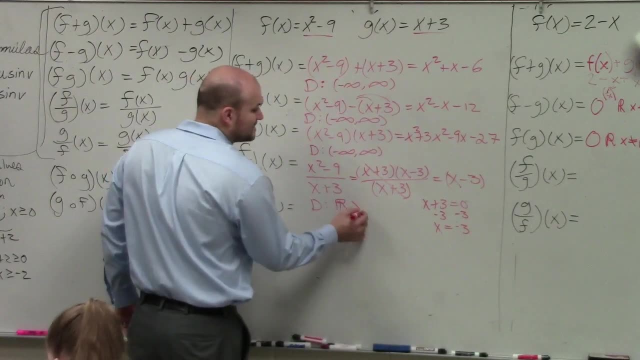 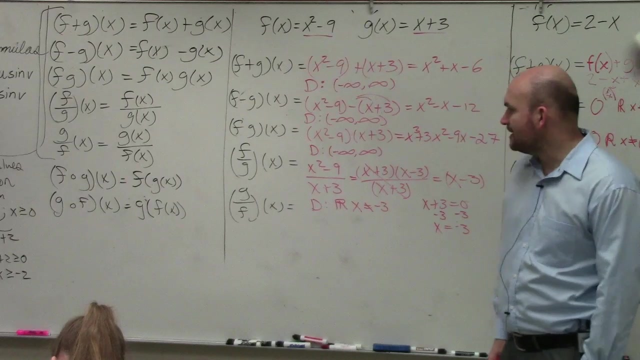 Just set your denominator equal to 0. That will tell you the values. that's going to equal 0, which is negative 3. So therefore, x- all real numbers except x- cannot equal negative 3.. All right, And then the last one is to do g of f of x or g of f of x. 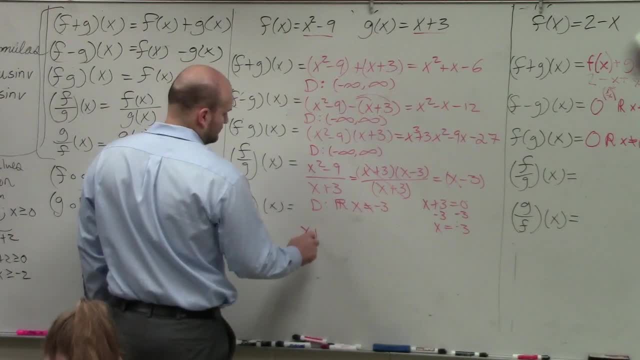 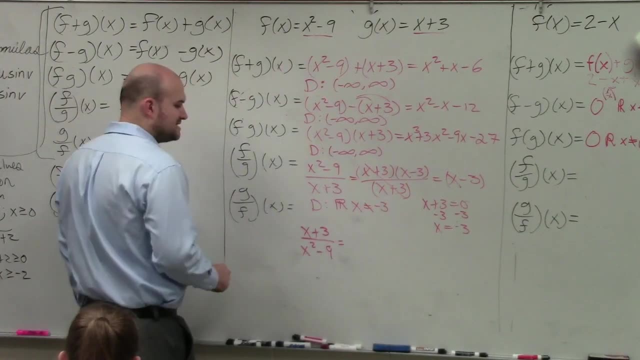 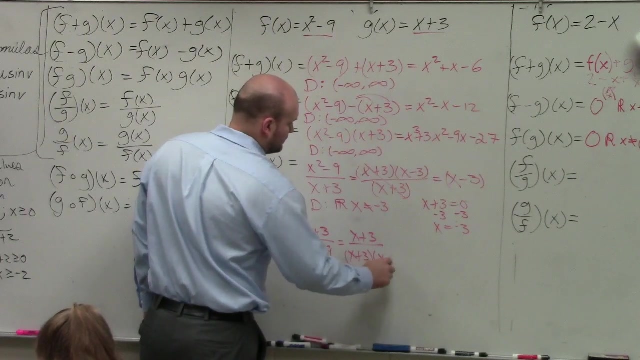 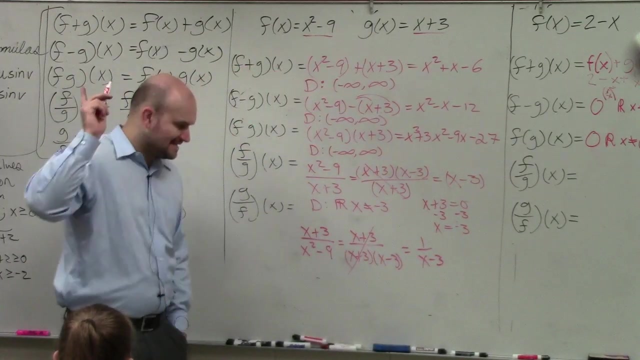 So now I do x plus 3.. Again, you can do the same thing: Factor it, Those, divide out, So I'm left with 1 over x minus 3.. However, as I mentioned to you, when you're identifying the domain, you 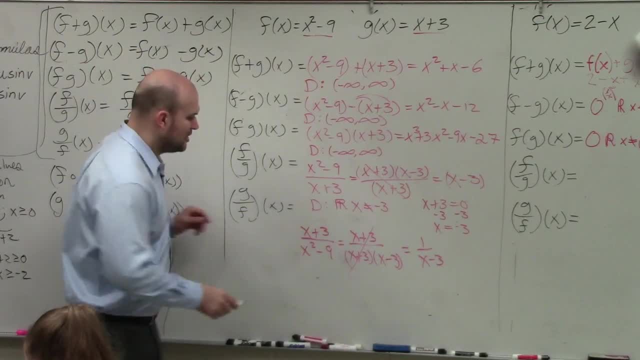 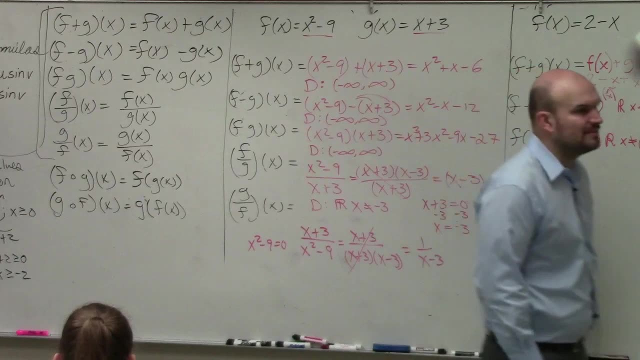 want to go back from your original answer, not your simplified answer. So all we would do is to find the domain. We'd set our denominator equal to 0.. Does everybody understand why I'm setting my denominator equal to 0?? The reason why I'm setting my denominator equal to 0.